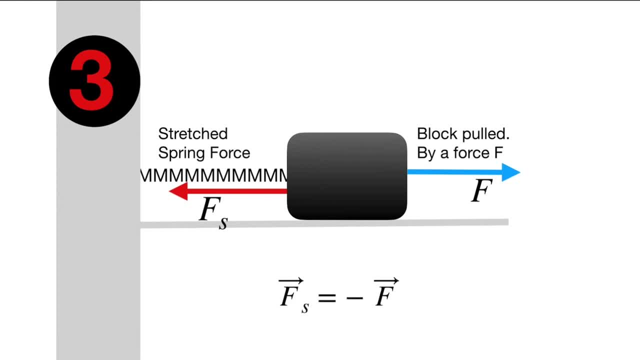 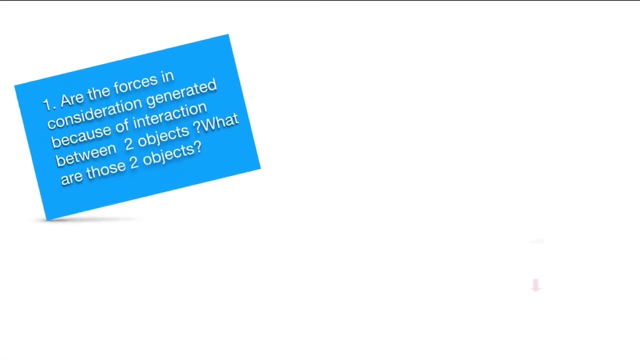 force works on the block in negative x direction. Is this pair of force F and spring force can be considered as Newton's action and reaction force pair? To answer these, ask following questions to yourself: 1. Are the forces in consideration generated because of interaction between two? 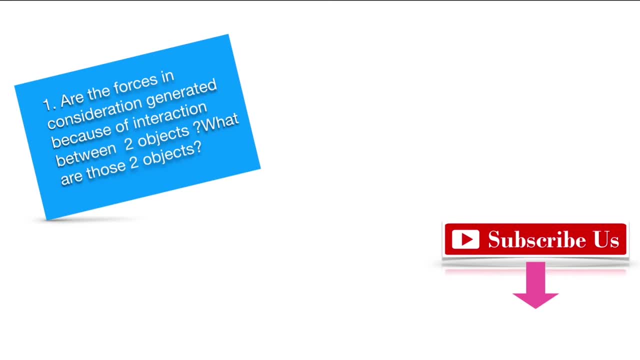 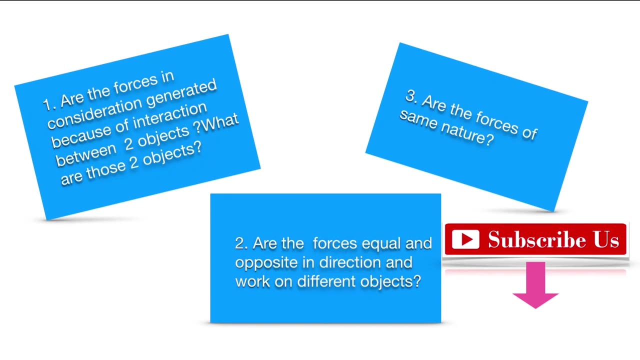 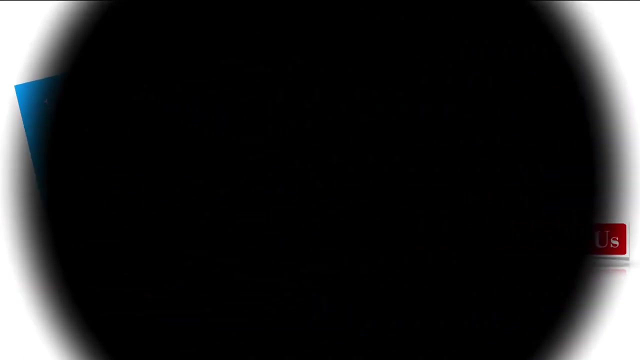 objects. What are those two objects? 2. Are the forces equal and opposite in direction and work on different objects? 3. Are the forces of same nature? Same nature means like gravitational force, spring force, normal force, etc. If answers to any of the above question is no, 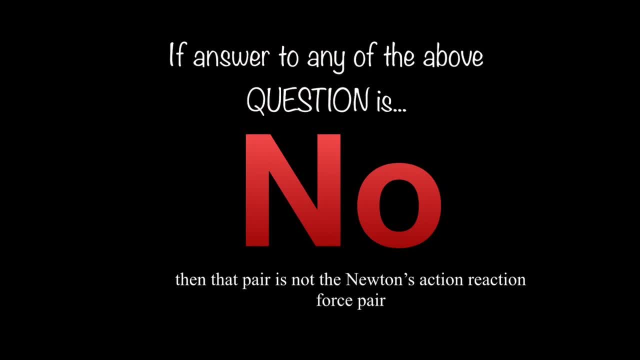 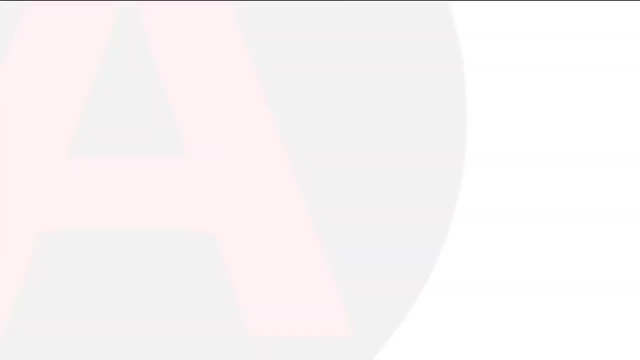 then that pair is not the Newton's action-reaction force pair. Now, before going back to these examples, let's check out few more cases. Case A: In a rocket launch, the rocket lift force is equal and opposite to the combustion exhaust. 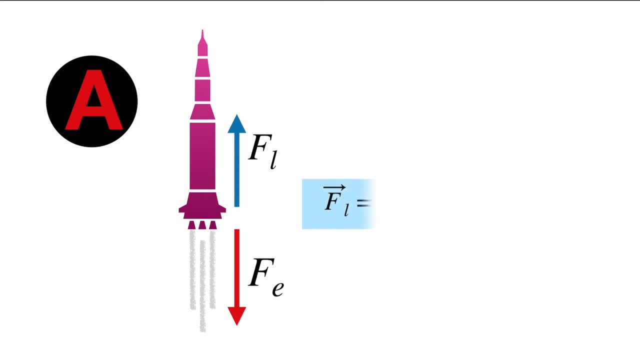 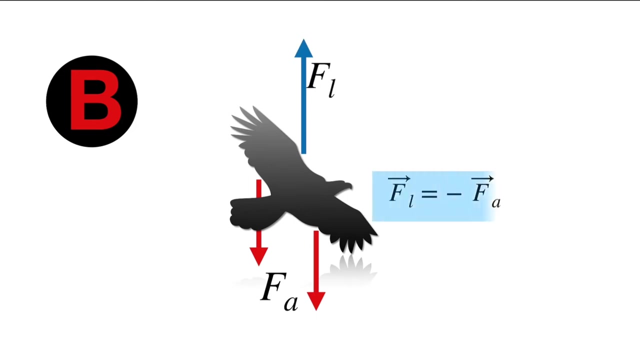 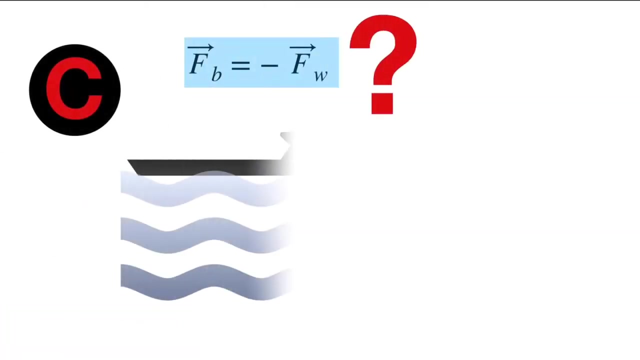 force. Do you think these forces makes Newton's third law force pair? Case B: A bird fly upward because of downward force, but it can't fly upward due to its wings. But can these equal and opposite forces be considered as Newton's pair of forces? Case C: What about equal and opposite forces during? 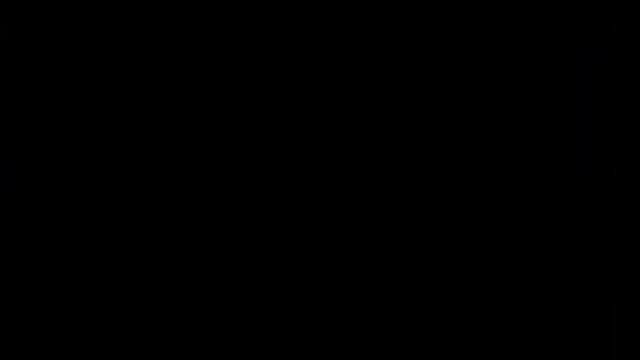 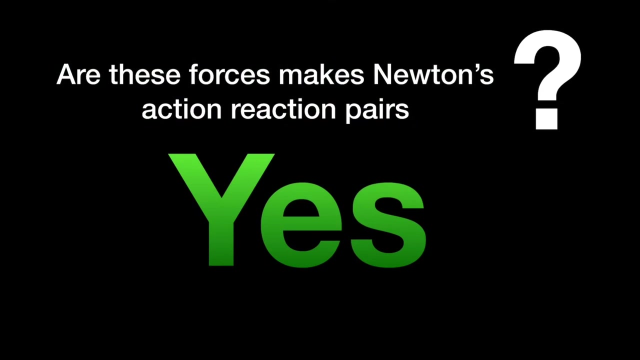 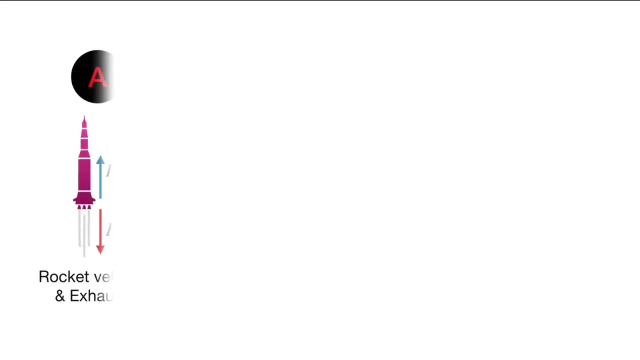 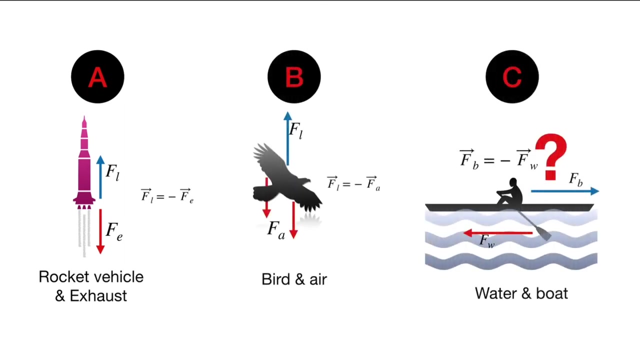 the rowing of a boat. Are these forces mate's? Newton's action-reaction pairs? Yes, In all the above three cases just discussed, forces are related to interaction of two objects: rocket, vehicle and exhaust, bird and air, water and boat, equal and opposite. 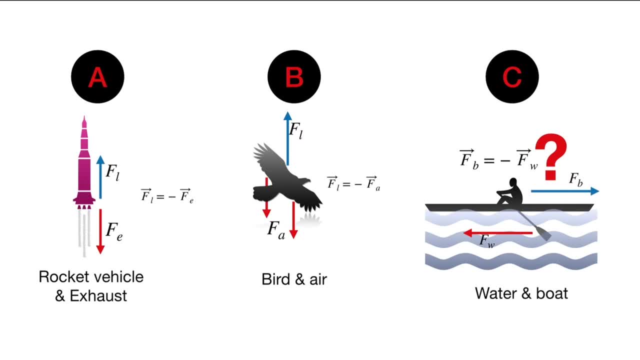 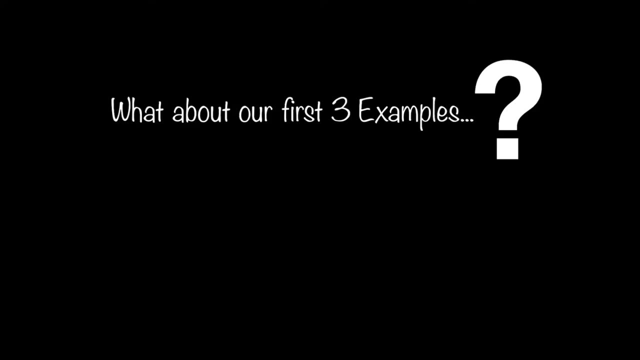 direction and are of similar nature. So those are Newton's third pair of action-reaction forces. Now what about our first three examples? Our forces in each of those examples are Newton's action-reaction force pairs? No, Although in each of those examples 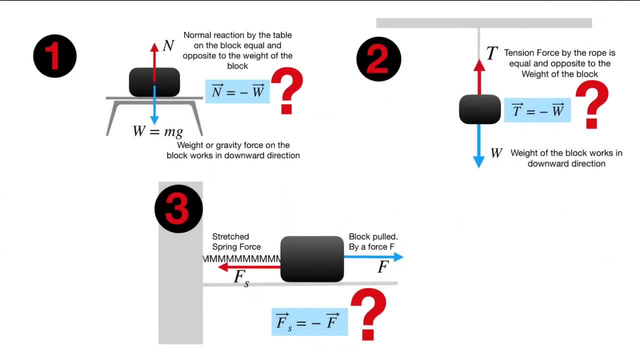 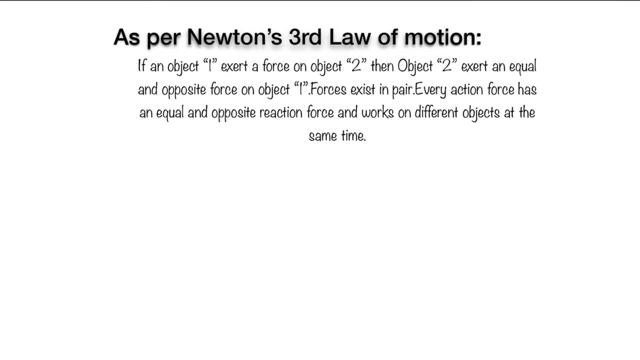 forces in considerations are equal and opposite, but they are working on same object block and not on the different objects. That's why they are not Newton's third law action-reaction pairs Now, as per Newton's third law of motion, since interaction force. 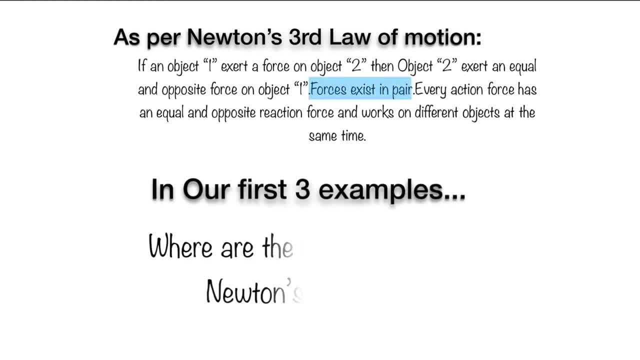 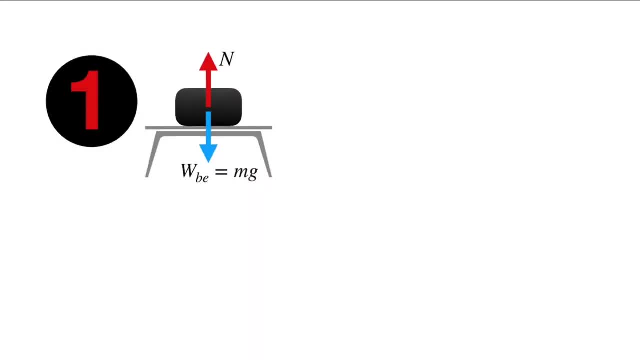 exists in pair. then, in our first three examples, where are the missing forces of Newton's force pairs? Example 1. There are two forces: weight of the block and the normal force. Weight of the block is gravity pulled by the earth on the block, toward its center And by the same force. 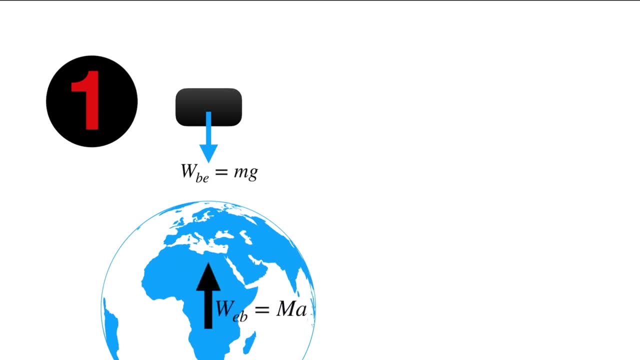 block pulls the earth in exactly opposite direction. Both of these forces are gravitational forces in nature and make Newton's third law of force pair. Now, what about normal force on the block Table exit: a normal force on the block equal and opposite to the block's normal force on the table in downward direction, In this case, normal forces. 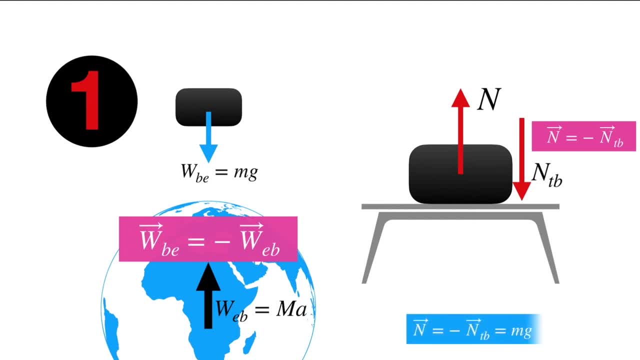 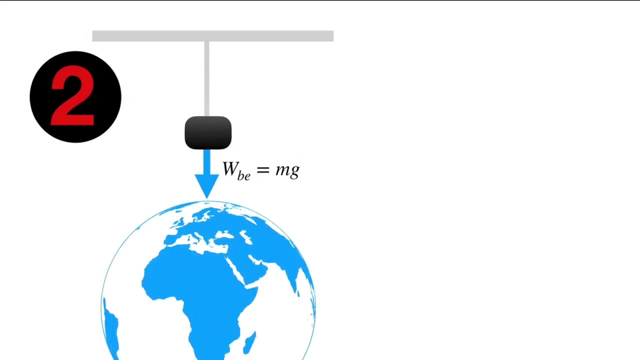 between block and table is same as block's weight, But it may not be the case when objects are in accelerated motion. We will see the effect of acceleration on the normal forces between two objects later in this video, Example 2.. Weight of the block is gravity pulled by the earth on the block. 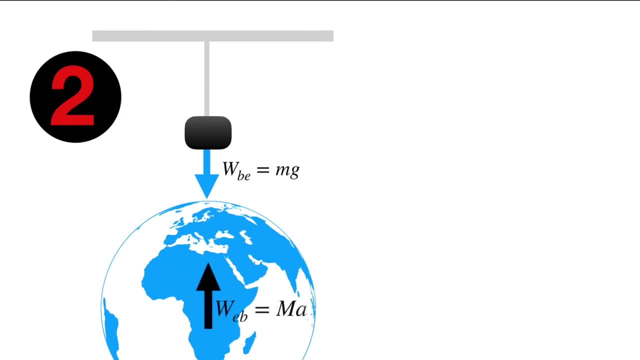 towards its center And by the same force block pulls the earth in exactly opposite direction, As we saw in previous case. both of these forces makes Newton's third law of force pair. Another force is upward tension force on the block. This is in reaction to the block's 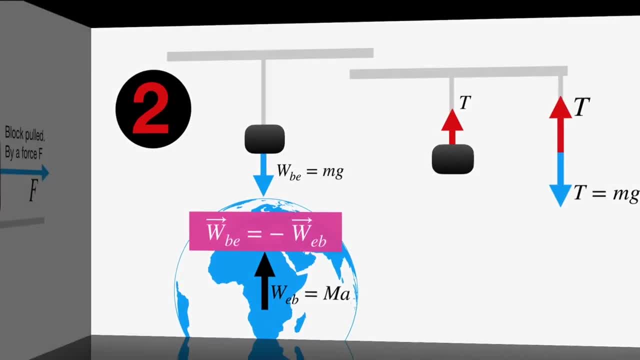 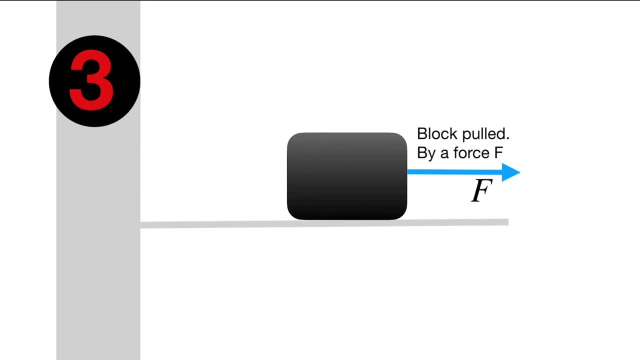 pull on the rope because of its weight. Example 3. Block pulled by a force, f exerts itself someone invisible. As a reaction, block pulls the invisible person by equal and opposite force: f? dash. So f and f? dash are Newton's third law of force. 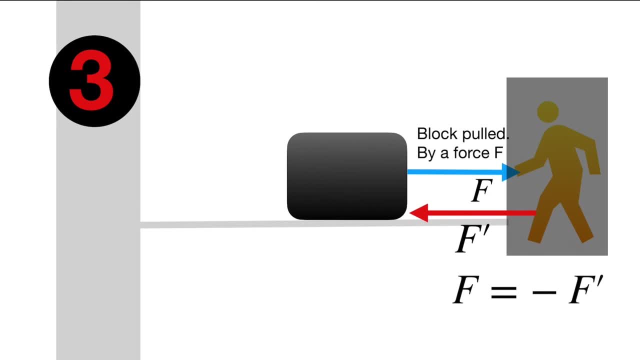 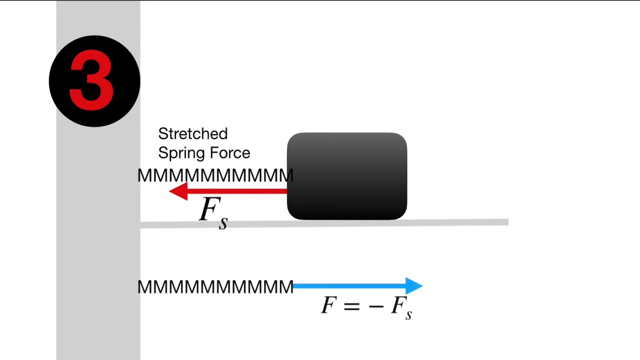 Let's work this out in 1, given bevoration chewy figured Easy way. First, a toda left occurs at one point. First the second left occurs at the left end of the corner of the top panel force pair. What about the spring force on the block? Block also pulls a spring with the same. 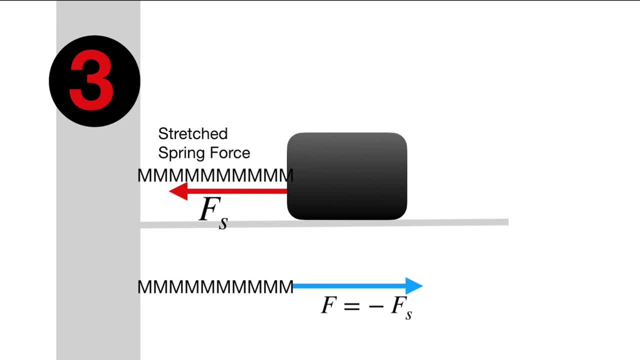 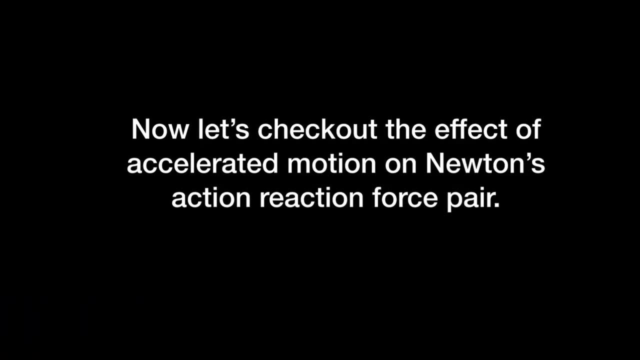 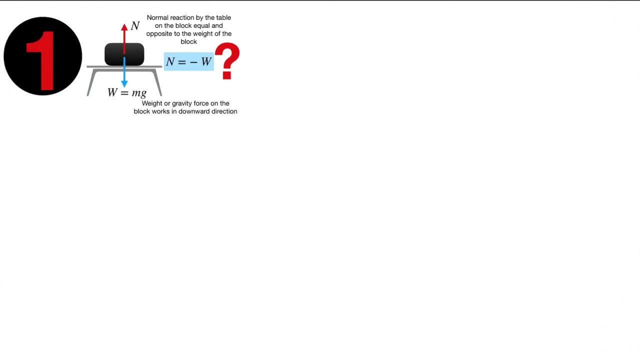 magnitude, but in opposite direction with force F. So F and Fs are the Newton's force pair. Now let's check out the effect of accelerated motion on the action-reaction force pair In example 1,. let's assume table and block are in accelerated elevator. 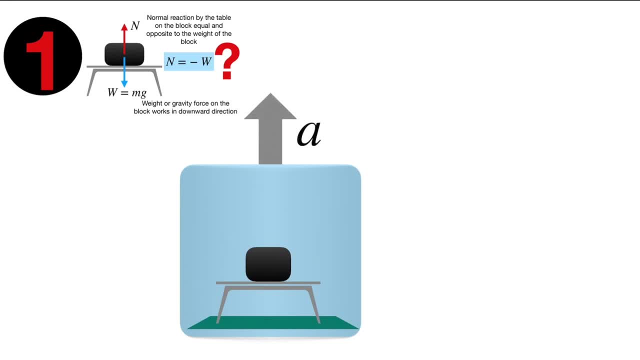 moving in upward direction with acceleration A. So in this case, what are the forces working on the block? Force of the gravity as weight, W in downward direction and the normal reaction force, N by the table, in upward direction. Now the block is moving with acceleration A. 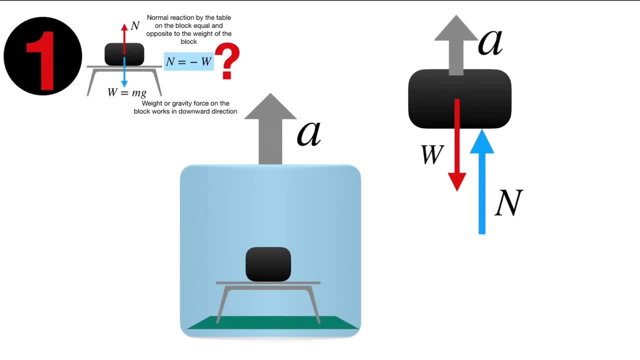 same as the elevator in upward direction. So, as per Newton's second law of motion, the net force is equal to MA. It shows that the normal force on the block increases by force MA. Now, at the same time, as per Newton's third law of motion, this normal force N by table. 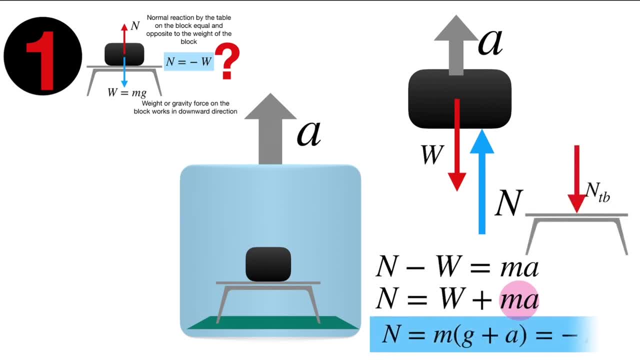 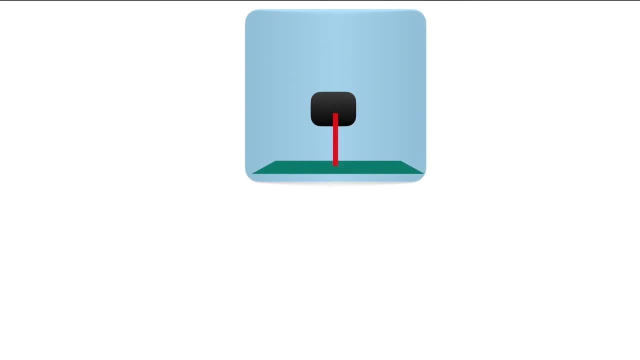 on the block is equal and opposite to the normal force, MA Tb on the table by the block. What about the gravity force on the block and its reaction force on the earth by the block? The earth gravity is constant near the surface, so its pull on the object remain constant, even the object accelerating in. 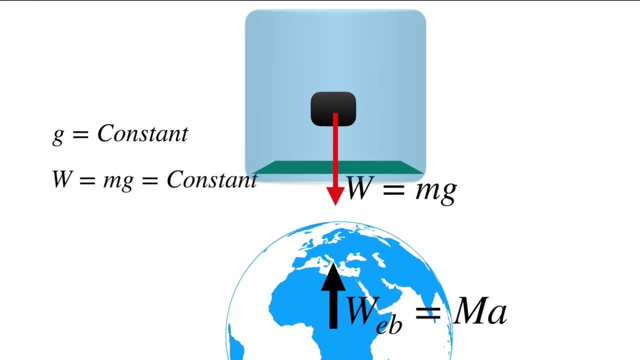 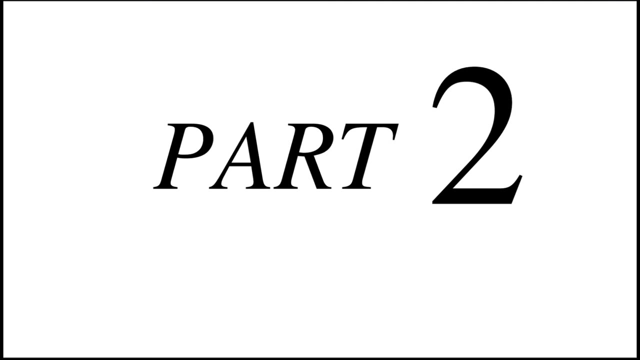 upward or downward direction? And what about the reaction force of the block on the earth? It will also same and remains constant. Check out next part of this video to know how to solve real-life problems using Newton's second and third laws. Before closing of this session, can you? 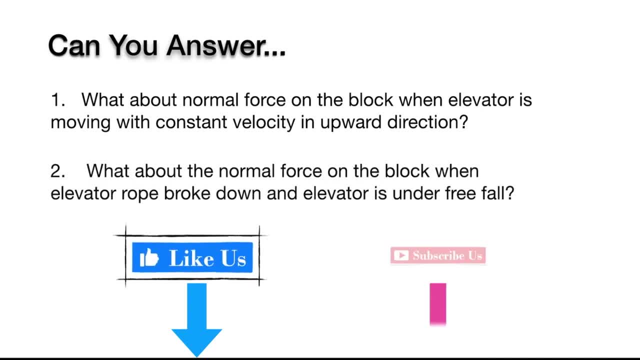 answer following questions. Put your answers, queries and doubts in comment box and let me know what part of this video you liked the most. Thank you, I hope you would have enjoyed this session. If you think you have learned something new today, then please click like button and subscribe us for similar. 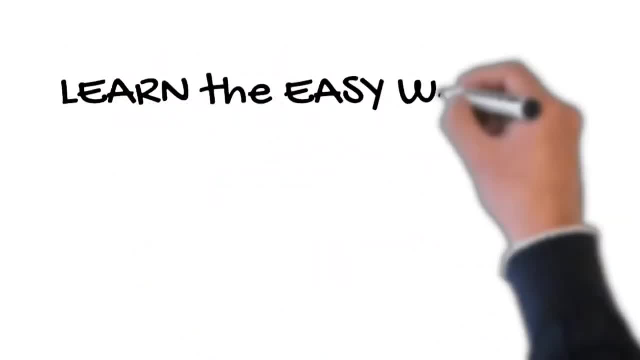 type of videos. Thank you for watching. see you next time. bye.